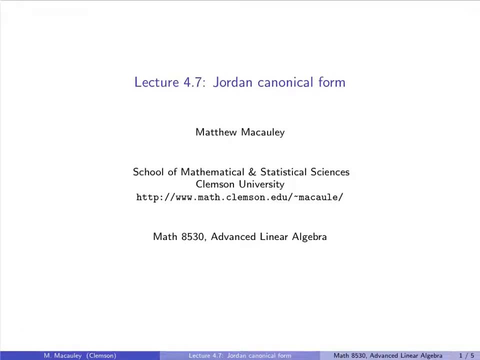 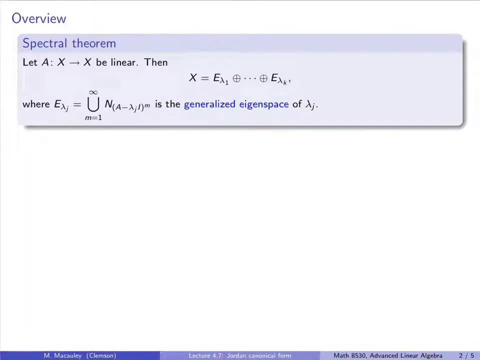 Welcome to Lecture 4.7, Jordan, Canonical Form. Let's recall the spectral theorem from the previous lecture: If A is a linear map of an n-dimensional vector space, then X decomposes as a direct sum of the so-called generalized eigenspaces of each eigenvalue. 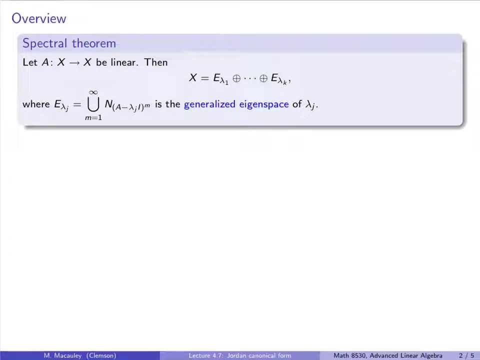 So E lambda j is the union of the null space of all powers, of A minus lambda j to the I. Now, if X is finite, dimensional, eventually this null space, these things grow as M gets bigger, but they will stabilize Now if we focus in on a particular generalized eigenspace: E lambda j. 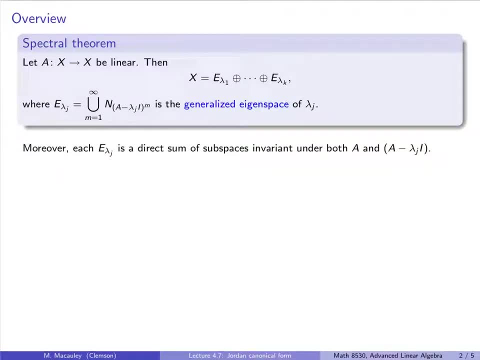 then that will be a direct sum of subspaces. These subspaces are invariant under both A and A minus lambda j I. Recall that a linear map is invariant under A if, and only if, it's invariant under A minus lambda j I, because this scalar times the identity doesn't actually really change anything. 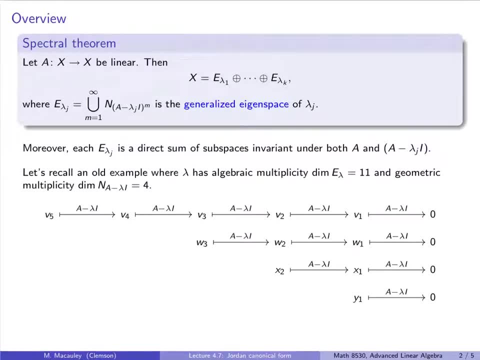 That's something that we proved a couple lectures ago. As I've been doing, I will recall an old example where lambda has algebraic multiplicity 11. That's the size of the generalized. There's only one eigenvalue and geometric multiplicity 4.. 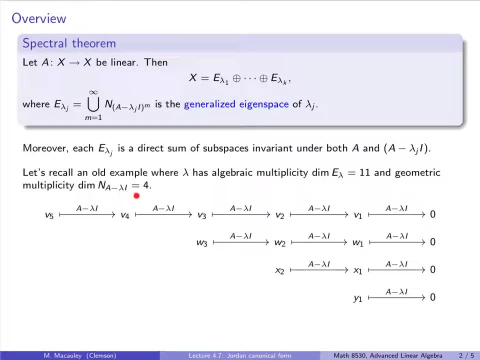 That means there are four eigenvectors. So recall this example. So here this is the null space of A minus lambda i. The null space is spanned by those four vectors. These seven vectors span the null space of A minus lambda i, squared. 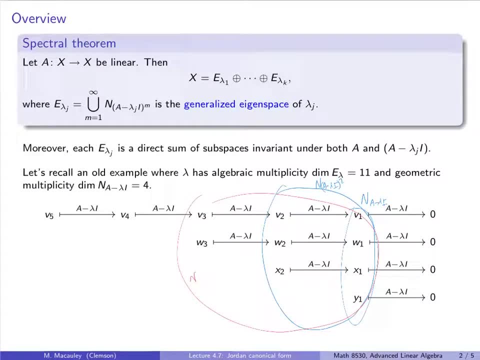 These nine span the null space of A minus lambda. i squared, i cubed and so forth, and so the the uh when i say that this is a direct sum of subspaces invariant under a and a minus lambda. i there, i am specifically speaking about these rows, so that 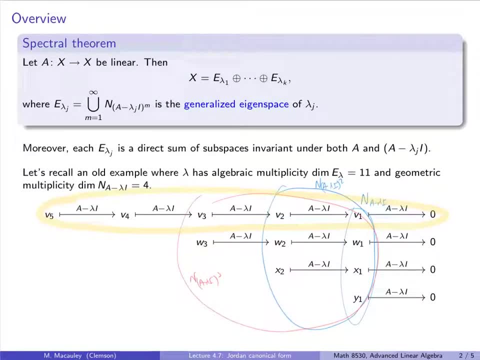 five-dimensional subspace, the one spanned by these is invariant under a and a minus lambda i. as is this- oops, let me get my highlighter back- as is this: this and this recall that if we have a vector space x that decomposes as a direct sum of subspaces y and z. 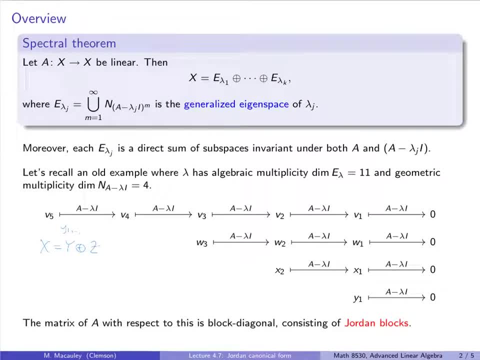 and we take a basis- y1 up to yk and zk, plus one up to zn, and we construct the matrix of a linear map, a, from x to x, then that basis, but then that matrix is going to be in block diagonal form. so we're going to have two blocks, one of them corresponding to the basis for y and the other 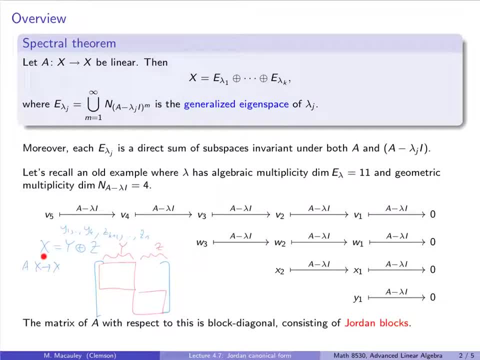 one corresponding to the basis for z and the basis for x is just the union of these two bases, and when i say block diagonal form, it's going to be zeros outside of these blocks. so, going back to this example, that means that we have a matrix of a and a minus lambda i and a minus lambda x. 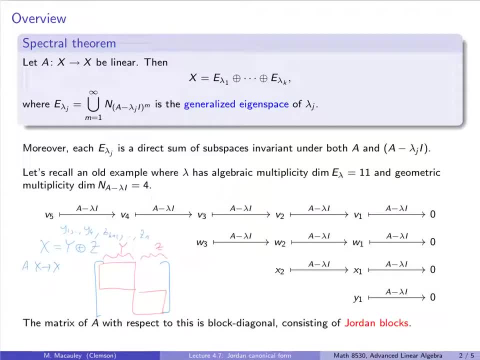 means that we will have a, so that the matrix of a is a is going to be 11, it's going to be 11 by 11 matrix, and if we pick these guys as the basis elements, then we then, in block form, what we're going to have is a 5 by 5 block, corresponding to this invariant subspace, a 3 by 3 block. 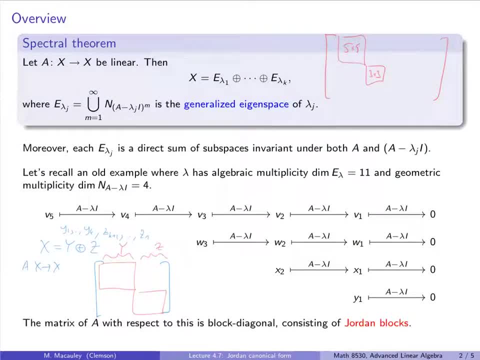 responding to this one: a 2 by 2, 2 by 2, and then a 1 by 1, and that is going to be. we've already talked about how. if you order a basis for these generalized eigenvectors- v1, v2 up to vk- then the matrix. 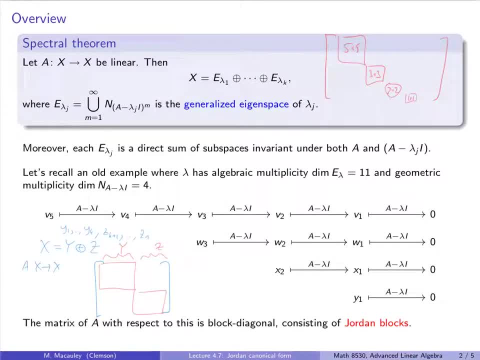 form for that is going to be a jordan block and the reason for that is because by construction, if we have v k, we apply a to it, then we get. you know, let me say, if we do a minus lambda i times vk, then we get vk minus 1, so a times vk. if we solve for avk up there, this is equal to lambda times vk plus 1. 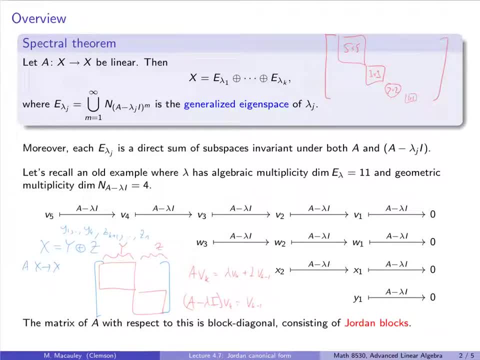 times vk minus 1. so remember how we construct such a matrix. we take our basis v1 up to vk and we apply a to it and then these these things here are are the columns of of the matrix. so the first column we're just going to have lambda times v1. the second column: 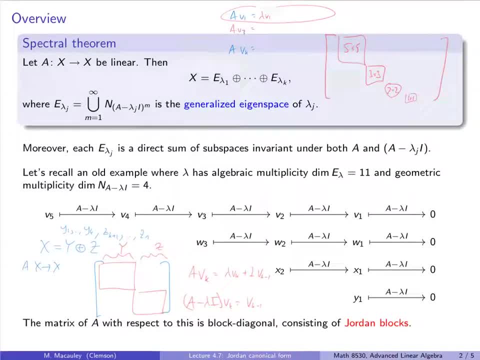 a v2 is going to be lambda, all right, i should say it's it's v1 plus lambda times v2, and then so forth. the last one's going to be vk minus 1 plus lambda vk. so notice how all of these columns are going to. 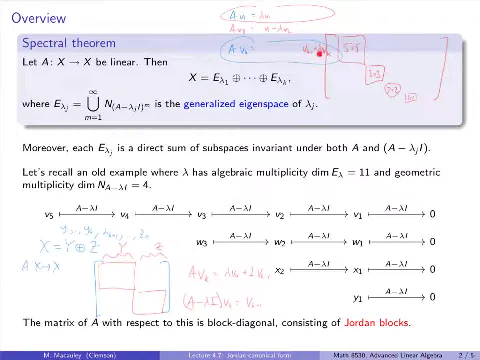 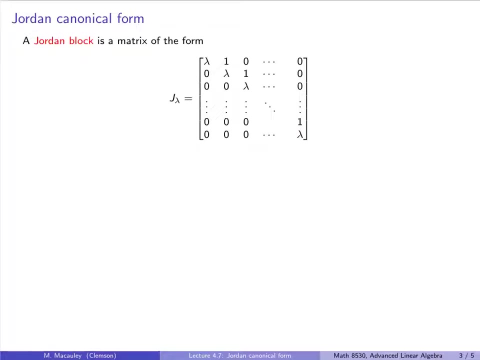 have, if you. this is the top, this is the bottom. they're going to have a lambda on the diagonal entry and then a 1 immediately above that, except for the first one, because there really is nothing above. so here is a jordan block, so it's just a matrix, a sub matrix that has lambdas on the diagonal. 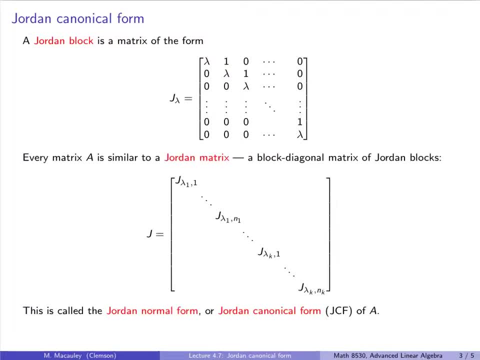 and it has ones directly above that. by the spectral theorem, every matrix is similar to a jordan matrix, a block diagonal matrix of jordan blocks. now recall that here i'm calling these. so all of these are blocks that refer to lambda 1, and then all of these down here are blocks that 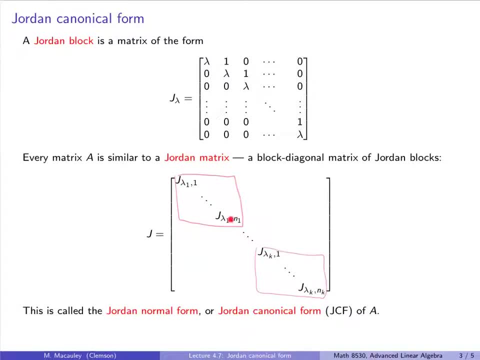 refer to lambda k. so think of this as like block, a block of blocks. and that's because, remember, by the spectral theorem, x decomposes as e lambda 1. the direct sum of these up to e lambda k and the eigenspace is either going to be a jordan block for each of. 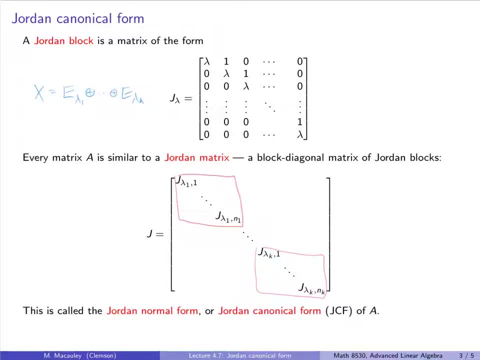 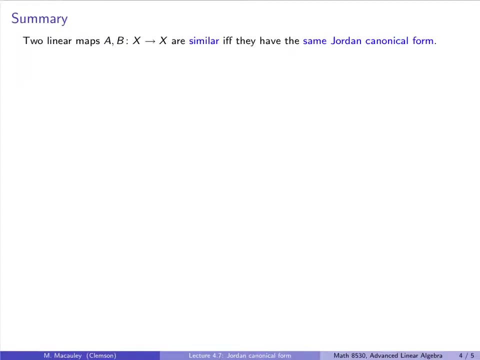 those so-called rows of eigen, generalized eigenvectors. this is called the jordan normal form or the jordan canonical form of the matrix or of the linear map a. we proved in the previous lecture that two linear maps, a and b, are similar if, and only if, they have. 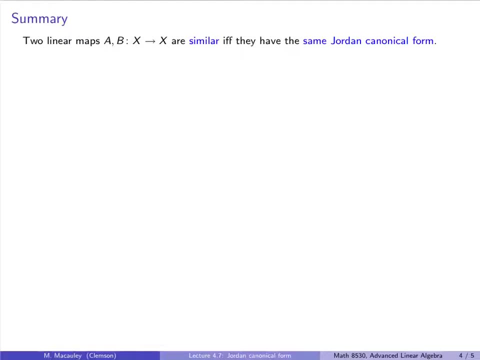 the same jordan canonical form. when i say they have the same, what i really mean is there is some way to order the eigenvectors, the generalized eigenvectors, so they have the same jordan canonical form, because if you reorder things, you reshuffle those chains and you're going to get 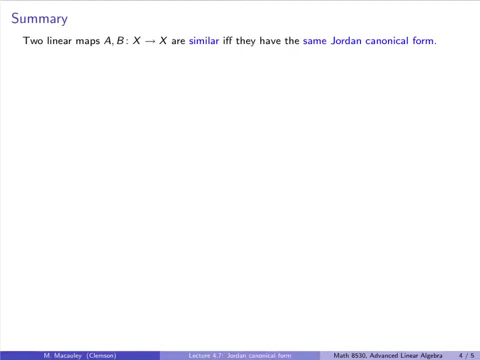 the same matrix, but you're going to just permute the jordan blocks. so now what i'm going to do is go back to some of our definitions about generalized eigenvectors and eigenvalues and characterize them. i'm going to summarize what we've learned, characterize them. 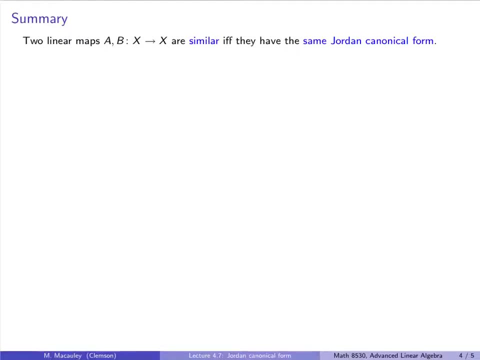 both in terms of polynomials, in terms of eigenvectors, geometrically and also in terms of jordan canonical form. now, i did this a few lectures ago, but that was before we had proven the spectral theorem, so i said it was a, i said it was a preview. this is when we do this. this is what we will be. 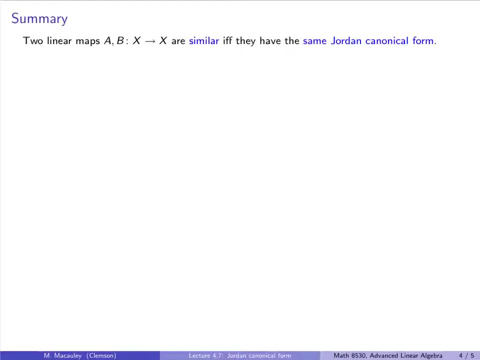 conclude, and even after we prove the spectral theorem, it i then had to prove that you don't have these generalized eigenvector chains that merge, so you don't have anything like that, or you know. you also don't have a eigenvector that's going to have multiple generalized eigenvectors. 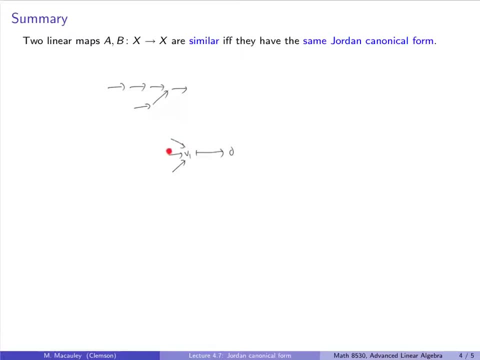 into it. well, i mean, i guess you can have multiple ones, but they're, they're, they're going to be equivalent in in some quotient space. so, um, look back to um, the spectral theorem that we did after that in a previous lecture, for why we eliminated these cases. 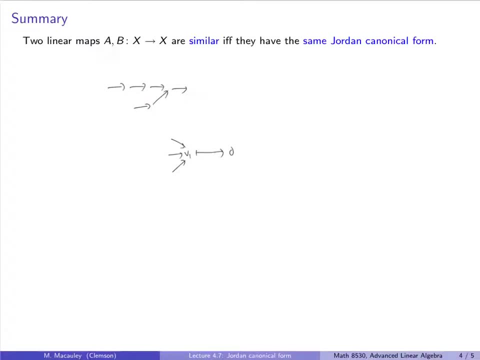 so i did say back in that original lecture that this is a preview as to what we we will learn, and hopefully it made sense. but now we can actually formally state these characterizations. so let's, let's get right to that. first of all, for each eigenvalue lambda, the algebraic multiplicity. 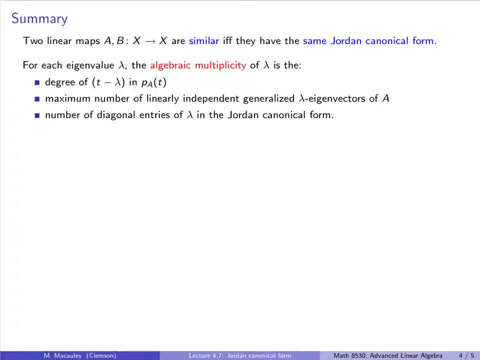 of lambda, often what you call the regular multiplicity. in your introductory, which is the near algebra course, it's just the degree of t minus lambda in the characteristic polynomial. geometrically it's the maximum number of linearly independent generalized lambda eigenvectors of a. so it's the if you take all of those, all the vectors that appear in this little chain diagram. 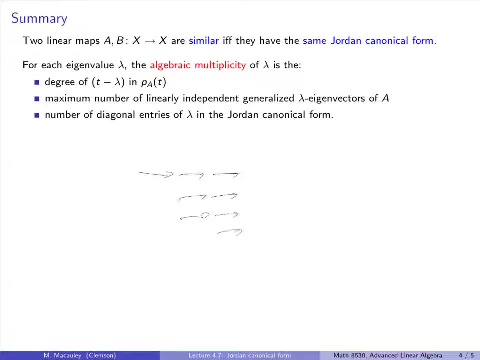 in any chain corresponding to to lambda, then that's the algebraic multiplicity and it's also the number of diagonal entries of lambda in the jordan canonical form, because each one of these things that that has, so let's put say this, is: v1, v2, v3, w1, w2, x1, x2, so forth. so each of these is 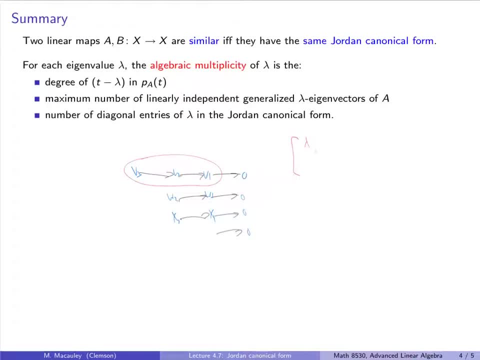 going to correspond to a three by three jordan block that's going to have lambdas on the diagonals. this is a two by two. so clearly, the number of diagonal entries is just the number of vectors that appears in this diagram. okay, that is algebraic multiplicity. next up is geometric. 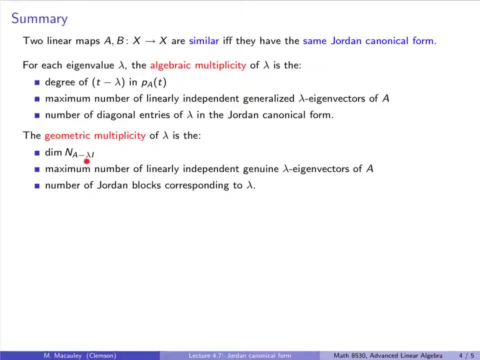 multiplicity. this is the dimension of a minus lambda i, which we can think of as the number of linearly independent genuine eigenvectors of a. and when i say independent, you know we say there's two eigenvectors but there's really infinitely many, because any combination is an eigenvector. but 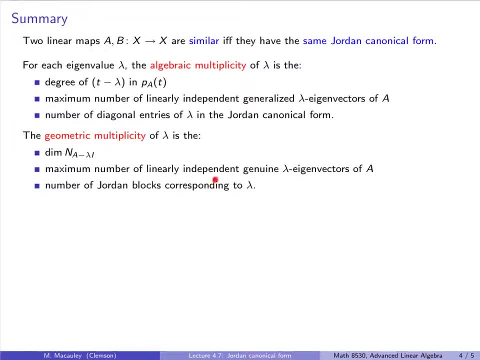 what's the maximum number of linearly independent ones in terms of our so-called chain diagram that i've been, you're probably sick of by now? it's the number of these, these chains, because you know, this is v1, w1, x1. what are the eigen, the genuine eigenvectors? they are these things, each chain. 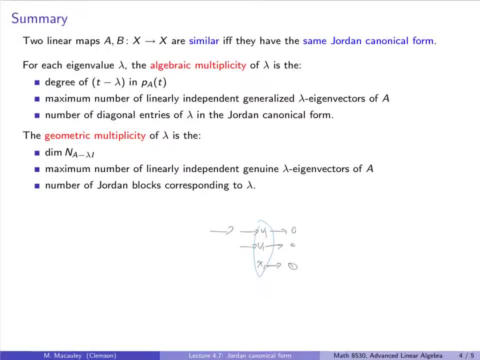 has one of them, it's the one that gets mapped to zero via a minus lambda i. this is also the number of jordan blocks corresponding to lambda, because for each of these chains- um, you know each of these chains corresponds to a jordan block and also notice why it's the dimension of a minus lambda i. 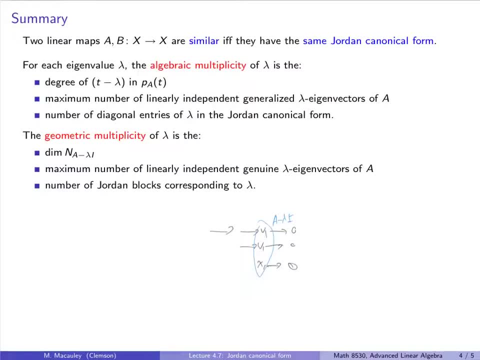 because the, uh, the null space of a minus lambda i. because you know what is that? these are the, those are the vectors that get mapped to zero right away. the index of lambda is the smallest d, such that nd plus one. remember where n, m is the null space of a minus lambda i to the m in terms of our chain. 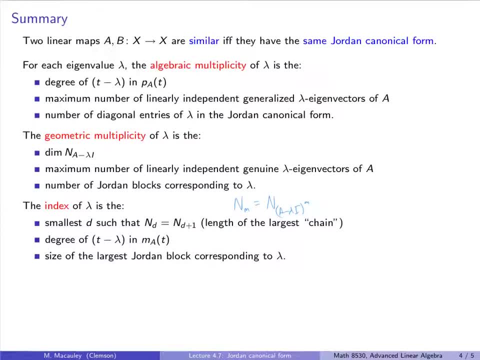 diagram. that's just the length of the largest chain. because if you get to the tip of one of these chains, if you have this chain going up here and you finally get to this, this vd, the fact that when it's equal to vd minus one means that if you go further, 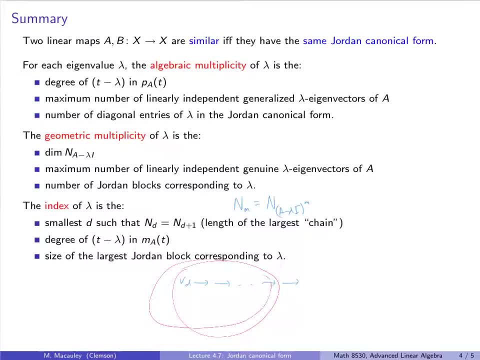 so this. so vd is all spanned by these, vd plus one. if you don't have any more vectors in there, then these null spaces will have not only the same dimension, they'll be the same. now remember that that's also the degree of t minus lambda in the minimal polynomial, because 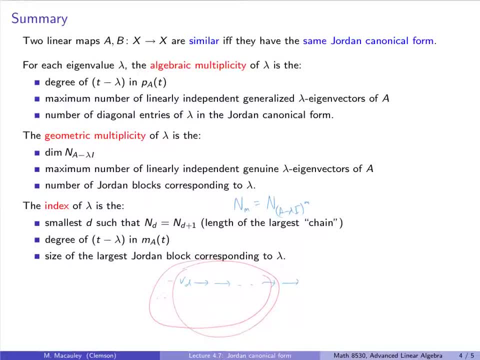 if you have a vd here which is a, which is d steps away from zero, you need at least a minus lambda i to the d iterations, or you need d iterations of a minus lambda i to send this all the way to zero. fewer than this won't work, so the minimal polynomial has to have this in it and more. 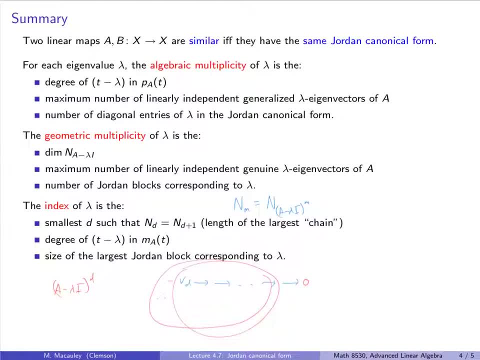 than it is not necessary, because this will do the trick. similarly, this is the size of the largest, largest jordan block, corresponding to lambda. finally, a is diagonalizable if well, by definition, it has a basis of genuine eigenvectors, or x has a basis. so remember. 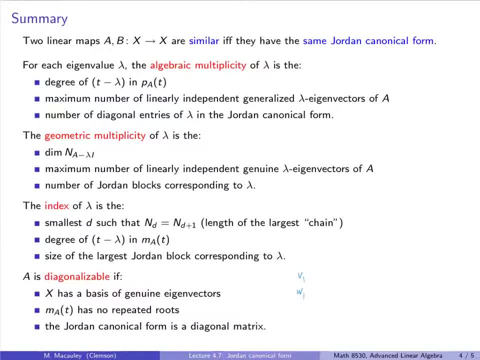 in terms of our chain diagram, that means that we have. so let's suppose it's four by four, that means that, with the basis for the entire space consists of eigenvectors that can map to zero. so that is equivalent to say that there is, there are no pre-images. there's. there's nothing. here's a. 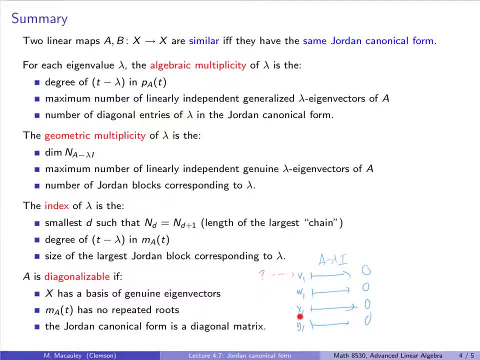 number of eigenvectors that get mapped onto v1 or any of these eigenvectors. that means that the minimal polynomial has no repeated roots, because you only need one eigen or one iteration of a minus lambda i for each eigenvalue. now this is the picture for lambda, but you might have. 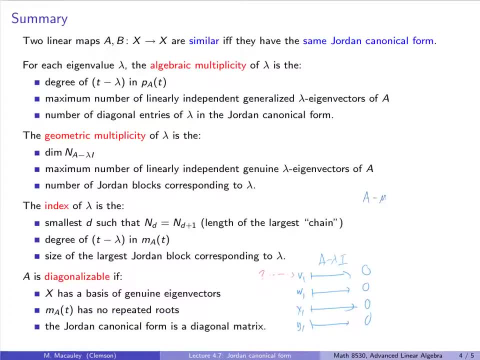 other eigenvalues, so you might have a minus mu. i has mapped some z1 to to zero and so forth. but if for every eigenvalue, each of these things has length one, then we don't need any repeated roots. we don't need a minus- lambda i squared- or higher for any eigenvalue to to kill off this. 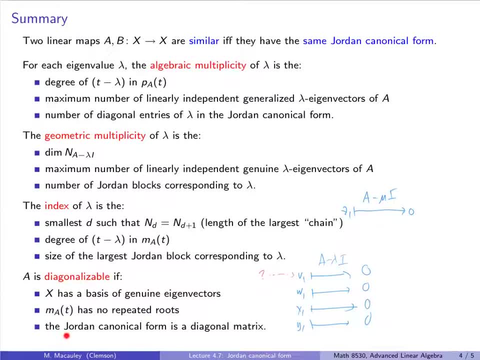 our basis of eigenvectors. finally, that means that the jordan canonical form is a diagonal matrix. in other words, a is similar to a diagonal matrix. so all of the jordan blocks are going to be um one by one, and that that's the square root of the matrix. so what we're going to do is i'm going to subtract a. 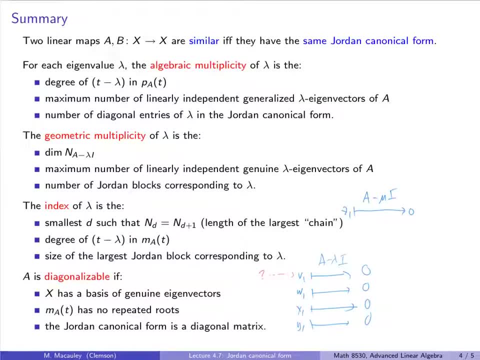 And that's what the word diagonalizable comes from- is that it's similar to a diagonal matrix. I know I've given this to you before, shown this to you before, but I really want to emphasize this diagram that you first saw in my lecture on change of basis. 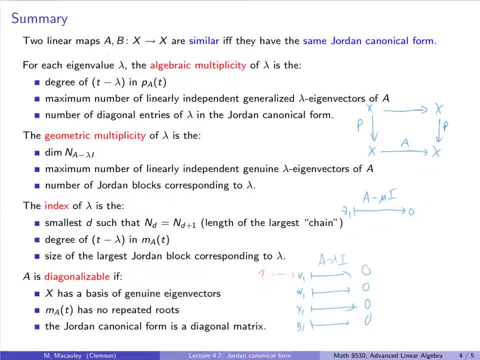 So that says that if you have a linear map A with respect to the old basis- E1 up to EN- then the change of basis matrix is V1 up to you. put the new basis in the columns and that's the thing that maps from here to top to bottom. 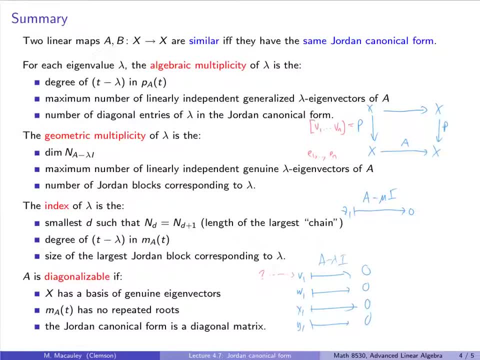 And so now this basis, this linear map up here, our basis is V1 up to VN. And so if you apply A to each of these- A up to V1,, up to VN- you get lambda V1.. You get lambda- sorry, lambda- 1, V1,. 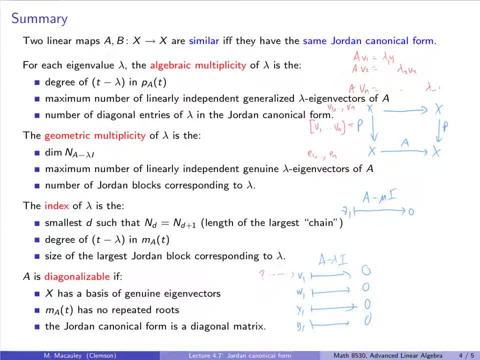 lambda 2, V2, up to lambda N, VN. So the matrix up here, here are the columns. It's literally a diagonal matrix. So D is equal to P, A P inverse. So do P then A, P inverse. 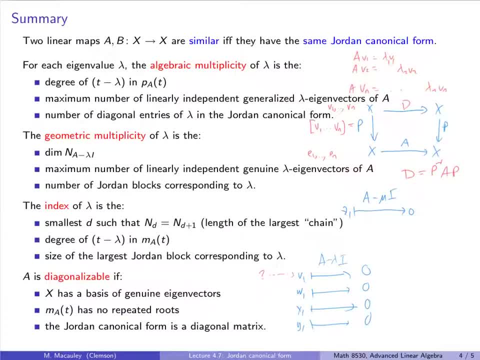 Reading right to left: P, A, P inverse. So I strongly recommend understanding this picture of these so-called generalized eigenvectors in the chains and also this change of basis picture and how. P is how the new basis up here. 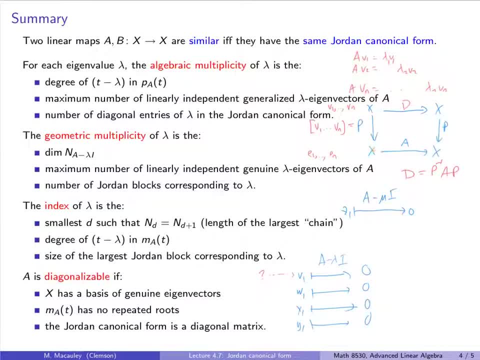 you go from the new basis to the old basis by a linear map or matrix P, where that new basis is in the columns. So understand these pictures. They will keep coming back and it'll really serve you well. You'll understand both of these things. 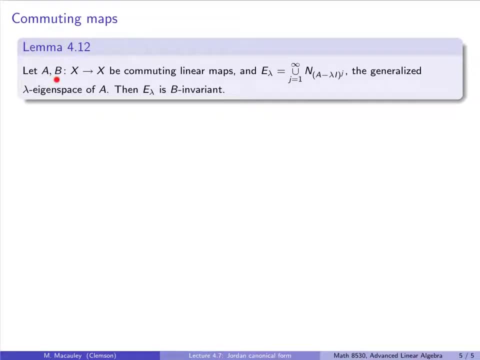 For the rest of this lecture, we will assume that A and B are linear maps on X which commute. In other words, A B equals B A. I'm going to prove several results about this. Well, actually one result. 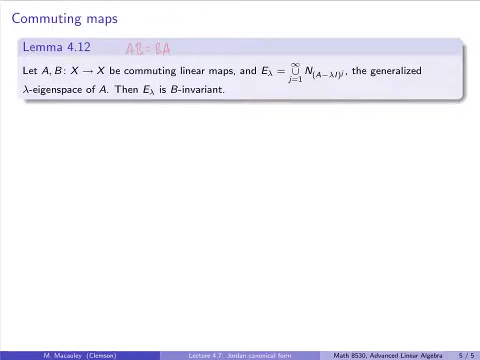 and then a specialization. But to do that we need this lemma: If we take an eigenvalue lambda of A and let E lambda be the generalized eigen space of A for that eigenvalue, so in other words the union of the null spaces. 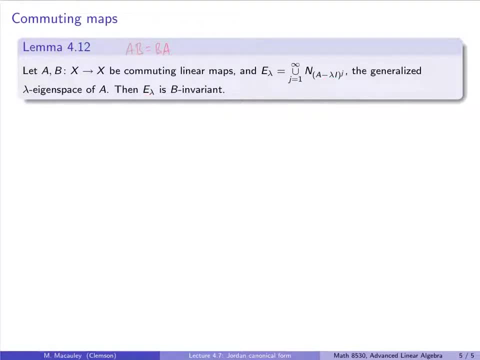 of all powers of A minus lambda I. then I claim that E lambda is also B invariant. We know it's A invariant, but I claim that it's B invariant as well. So, in other words, X is as a direct sum of the A eigenspaces. 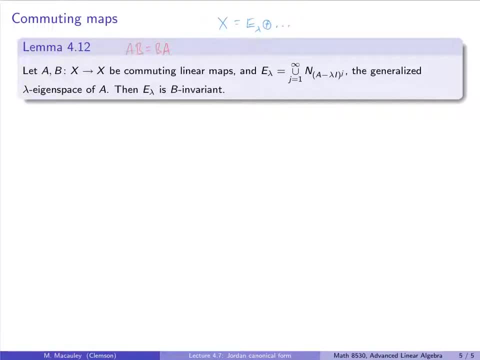 E lambda and then some other things. So what this says is that if we restrict B to E lambda, then it sends E lambda to itself. Now, I'm not a huge fan of this restriction. I think it's perfectly fine to just say: 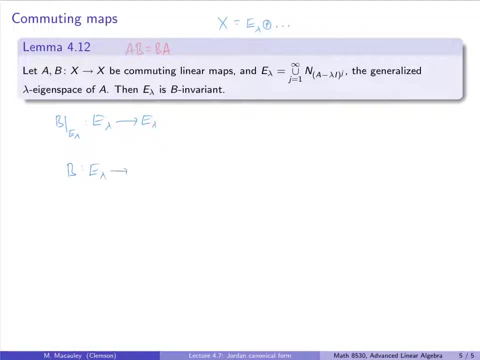 take B and sends E lambda to itself, And I think that the restriction is implied. I don't think we needed this extra nonsense here, So I'm just going to use this notation And let's think about why this is true. So E lambda literally is the set. 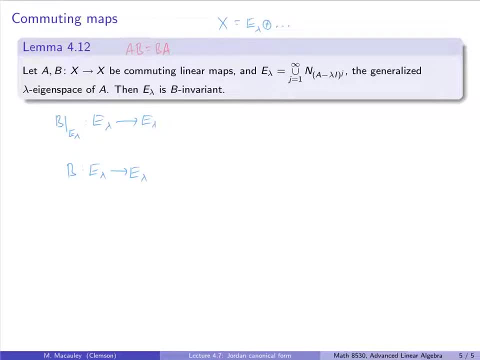 of all generalized eigenvectors of A corresponding to lambda. So if we take any, so let's take. so here's the proof of it. Let's take any X in E, lambda, then, by definition for some integer M, some nonzero integer M, 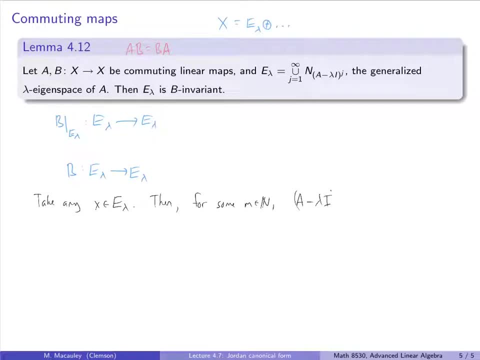 A minus lambda I to the M times X equals zero. That's what it means for X to be in this generalized eigenspace. It's a generalized eigenvector, Even if it's a linear combination of multiple basis elements from this generalized eigenspace. 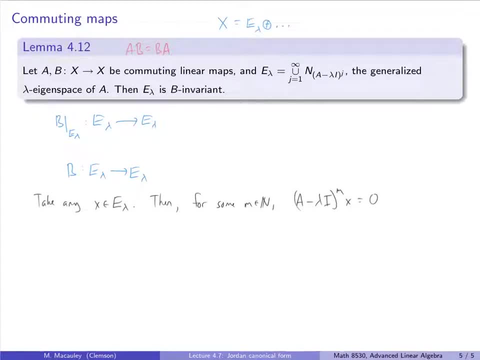 it's still a generalized eigenvector. So to show that B sends this space to itself, it's still a generalized eigenvector. I mean, in other words, B of E lambda is contained in E lambda. We just need to show that B of X is still a generalized eigenvector of A. 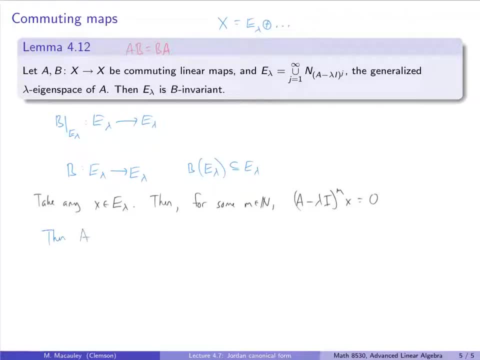 So then, A minus lambda I to the M times BX. We just have to show that that is equal to zero, And I claim that we can commute A. and I mean, I probably don't need to verify this, but let me just do up here. 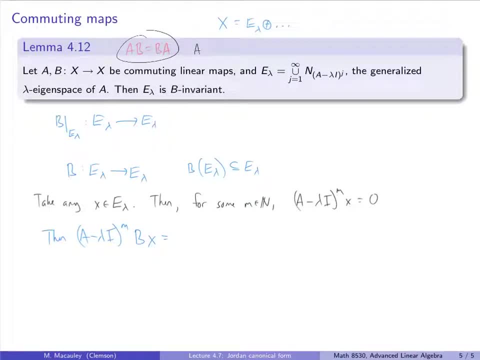 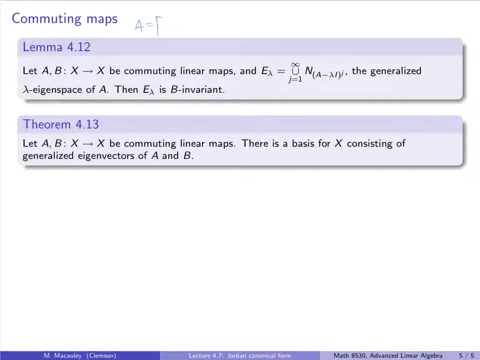 So I can take this and I can swap the B and the A minus lambda I to the N. So I can take this and I can swap the B and the A minus lambda I to the N. So, for example, if we take A to be the matrix 2,, 2,, 1, or so I guess 2, 1,, 0,, 2,. 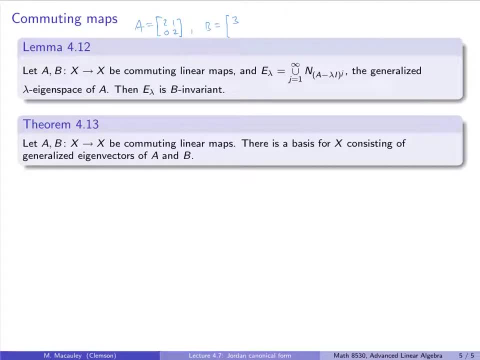 and we take B to be the matrix 3, 0,, 0, 3, then A is not diagonalizable. It has two, it has an eigenvector 1, 0.. It gets mapped 2 to 0 by A. 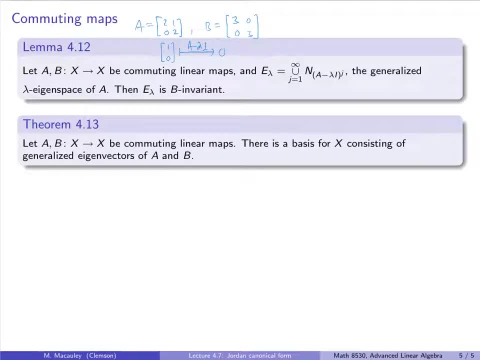 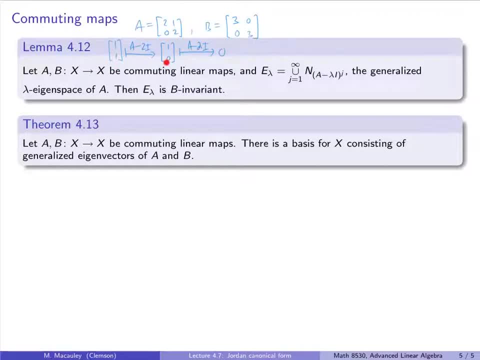 So here is a basis of generalized eigenvectors, And we don't have really too much room to choose here. So any eigenvector has to be a scalar of this, and then that's going to determine what this thing is. So let's call this thing V1. 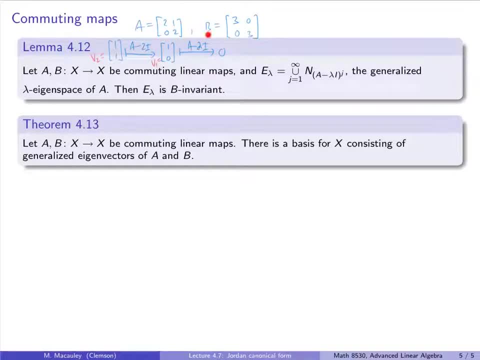 Let me call this thing V2.. Now B: if I were to ask you to find the eigenvectors for B, you would most likely just come back and say: oh well, let's take 1, 0 and 0, 1.. 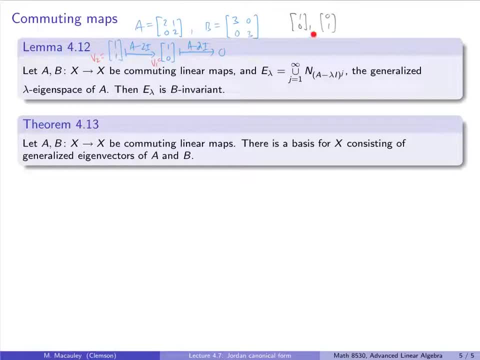 And you would be right. This is a linearly independent set of eigenvectors. That's the basis. But really every vector of X is a basis because this is a diagonal map. So for any vector, BV equals 3 beta. 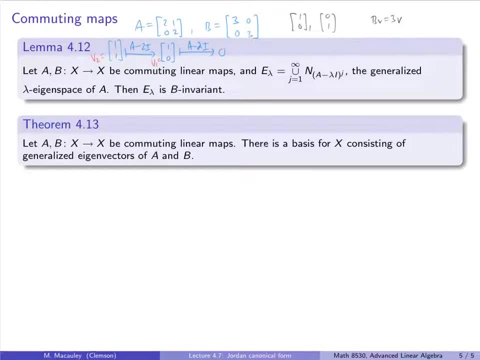 It's a diagonal matrix. So what I can't do is just take this basis, just take any basis, and say: well, these are eigenvectors of B, so they will be generalized eigenvectors of A. No, so we are forced over here to pick this for V1 and this for V2.. 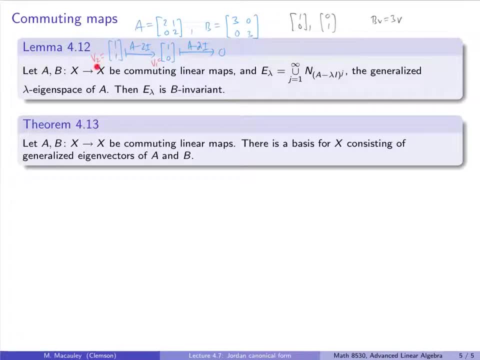 But because A and B commute, these things are going to be generalized eigenvectors for B and they will also be genuine eigenvectors. So these two vectors are the things that do the trick in this case. So notice that B is diagonalizable. 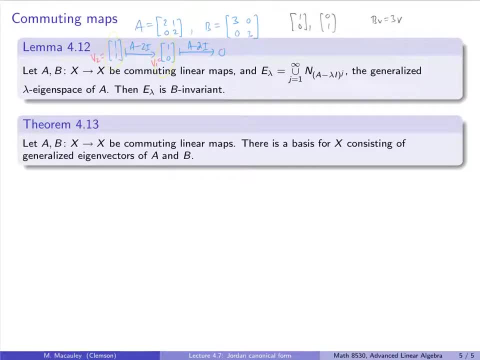 It's diagonal and A is not, So this is not saying anything. The Jordan canonical forms have a very different block structure, and you can imagine how different this can get for larger matrices. Okay, so let's prove this. We will start by writing X. 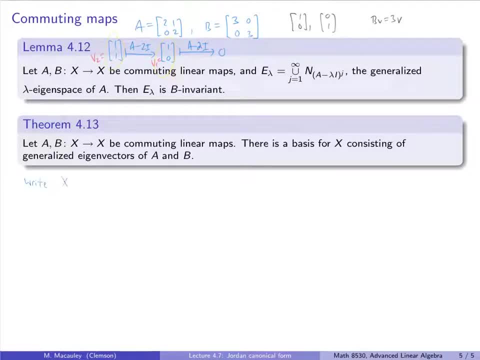 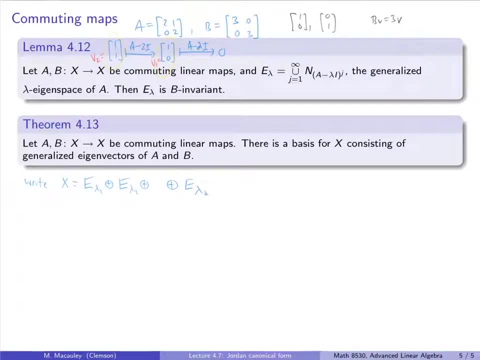 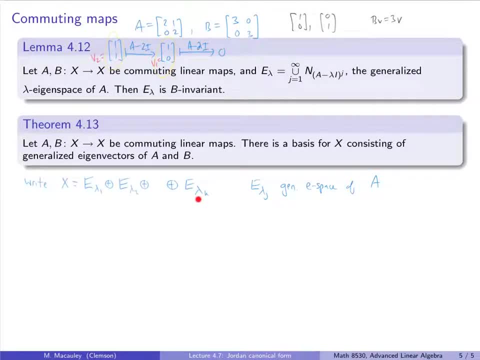 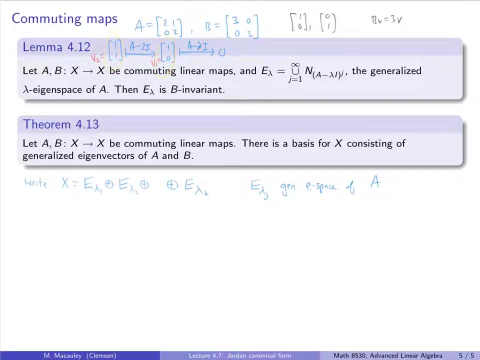 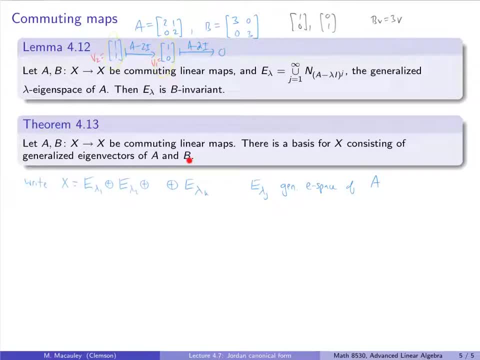 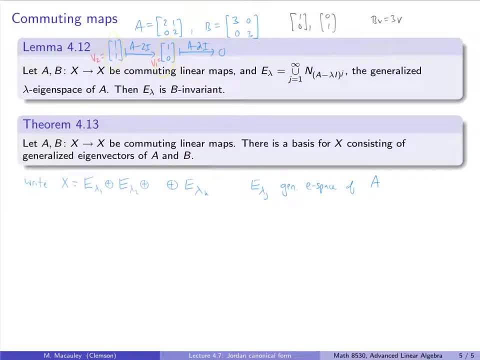 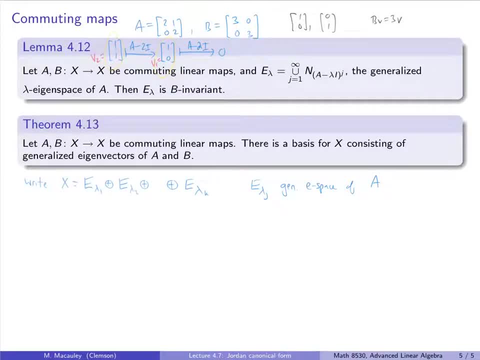 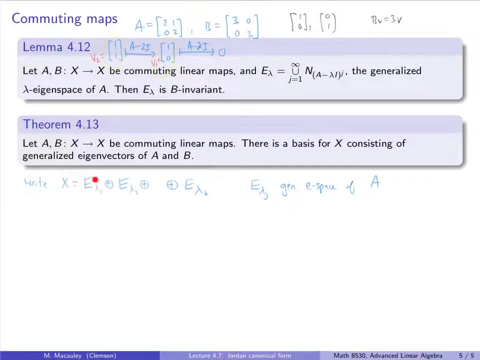 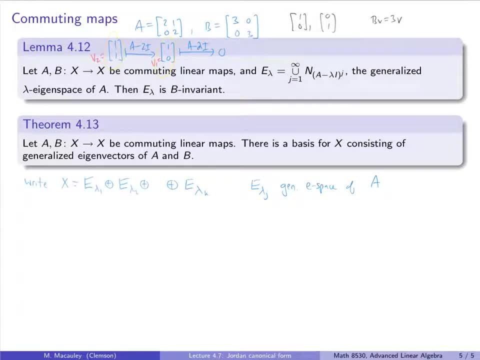 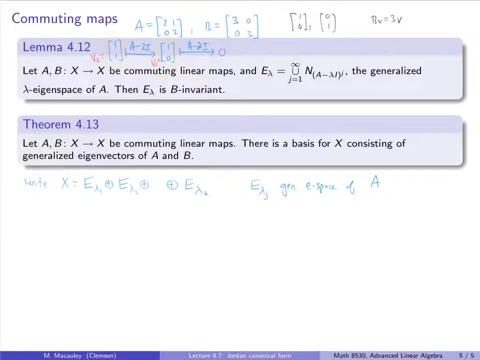 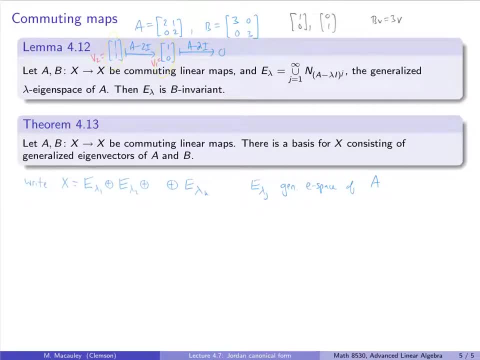 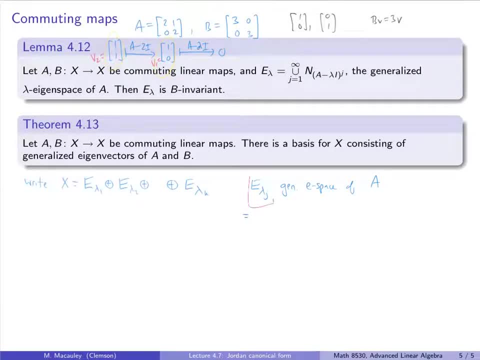 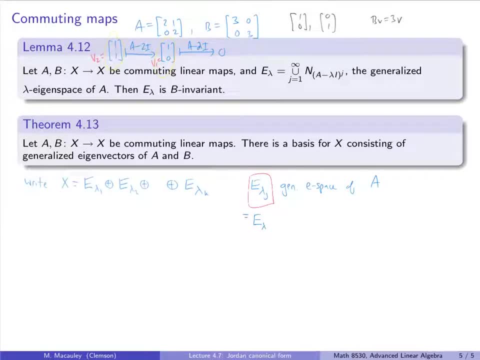 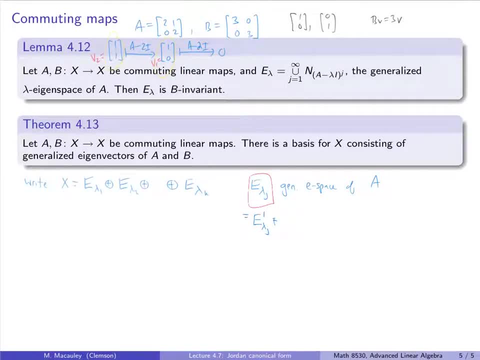 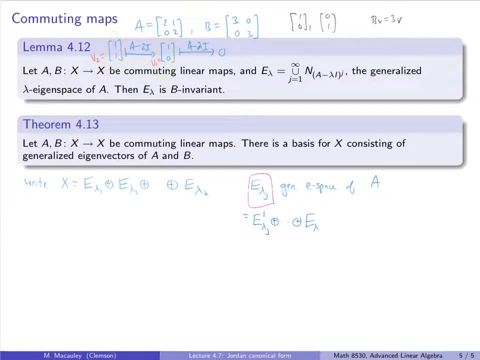 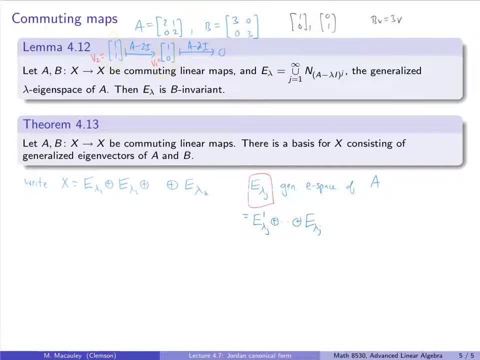 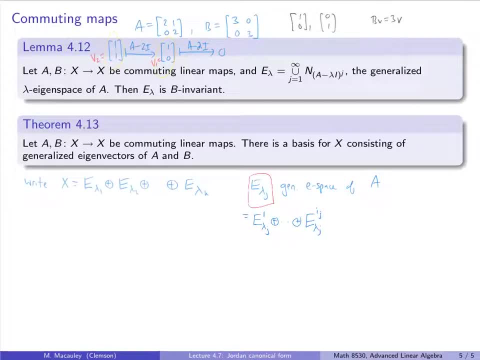 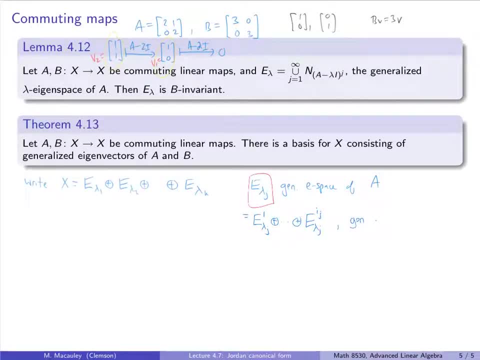 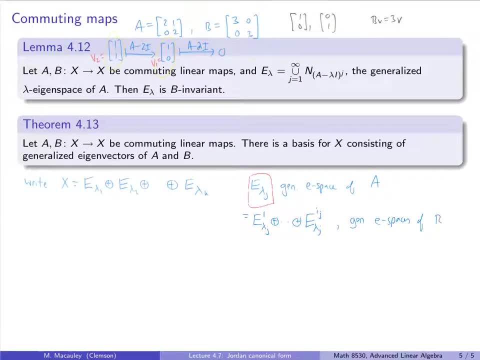 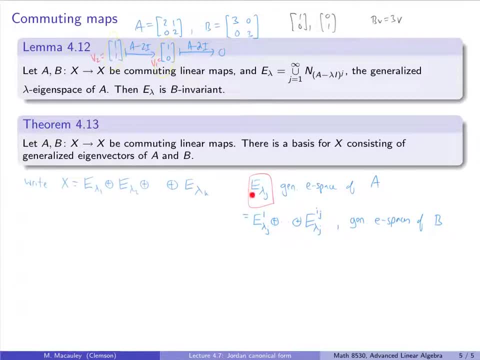 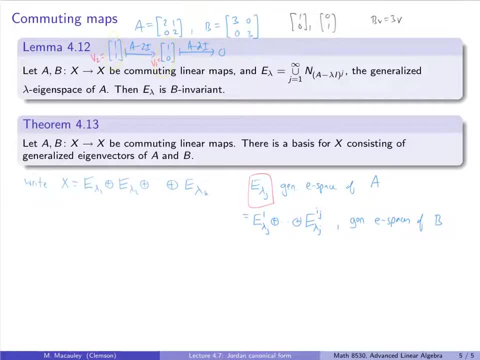 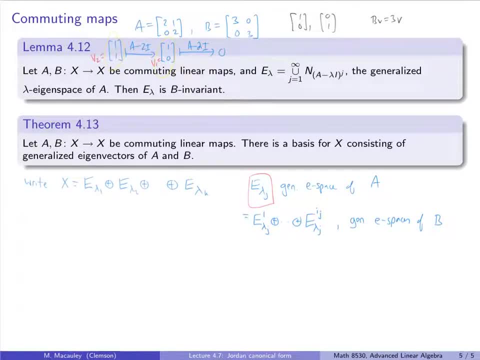 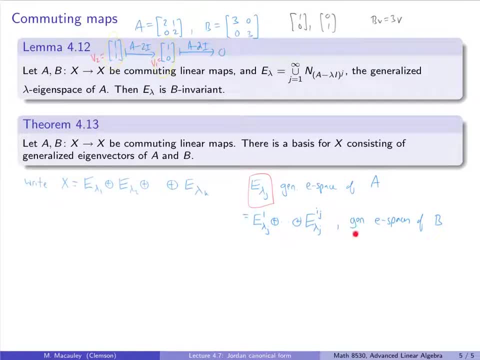 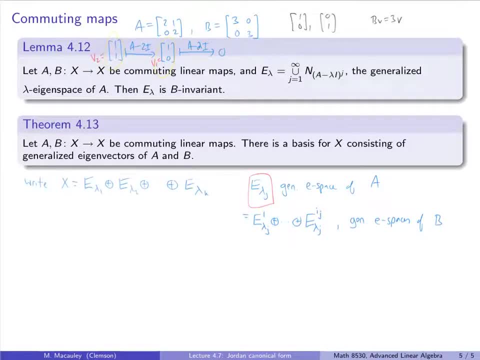 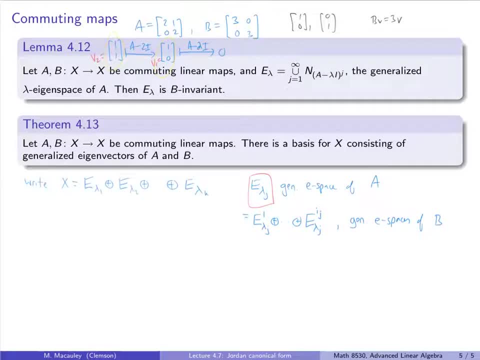 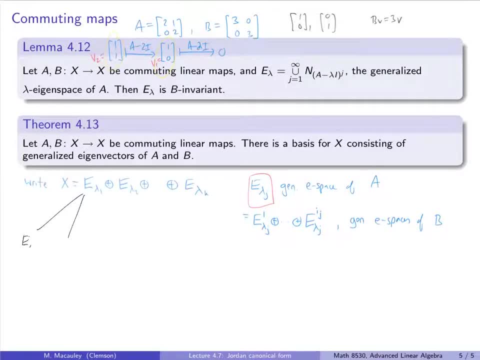 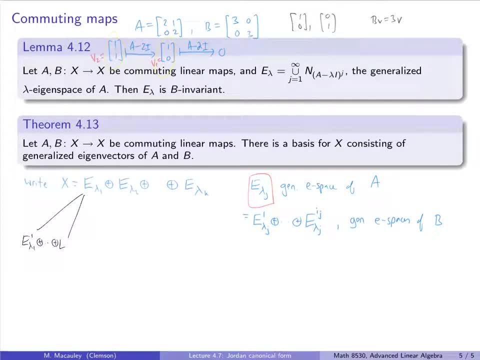 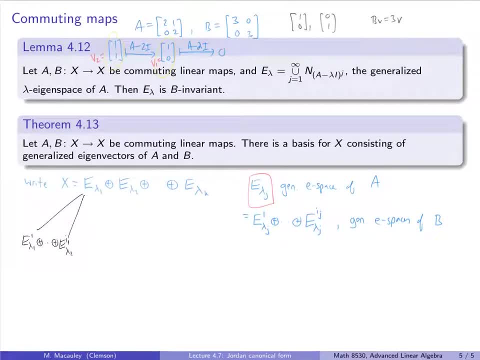 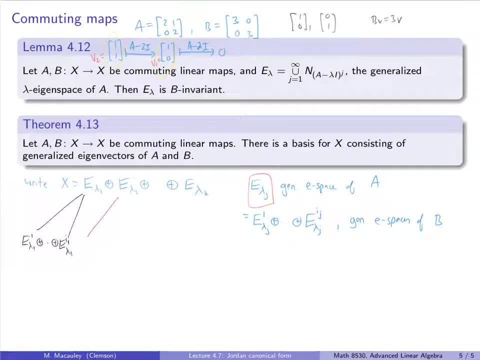 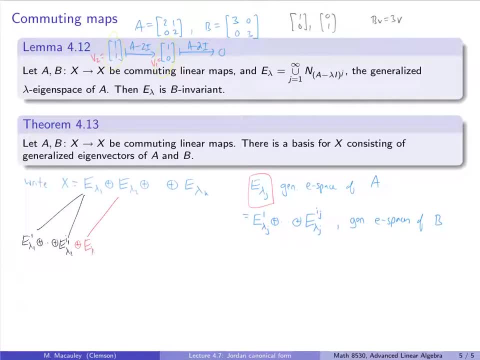 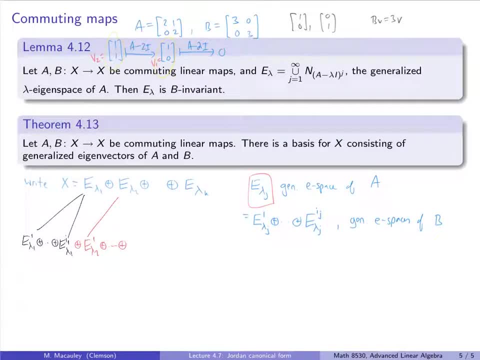 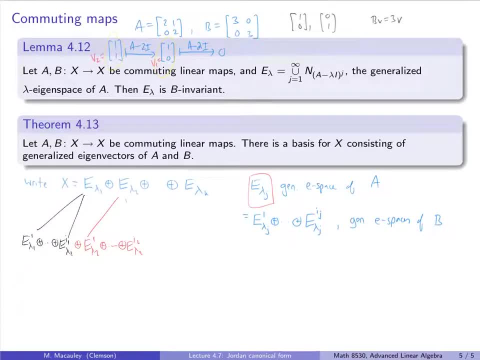 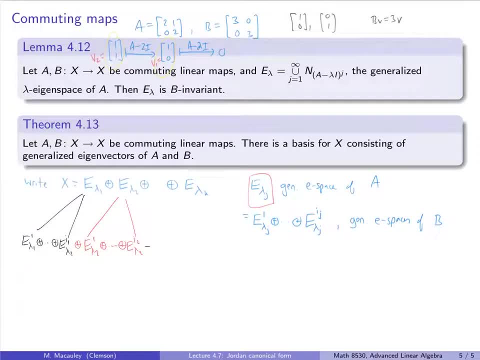 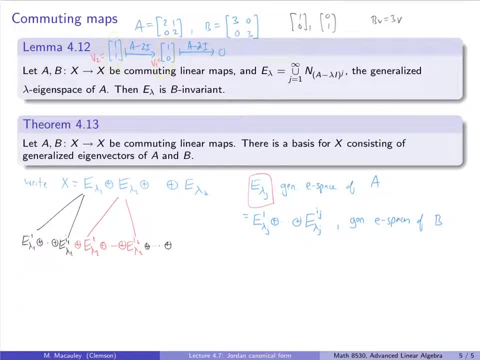 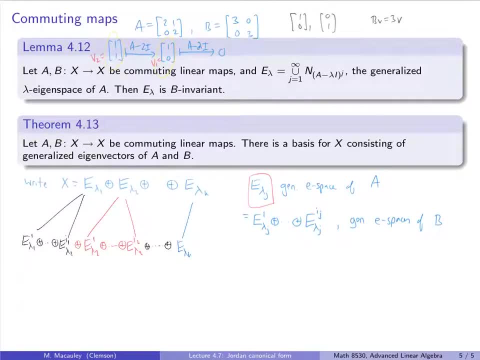 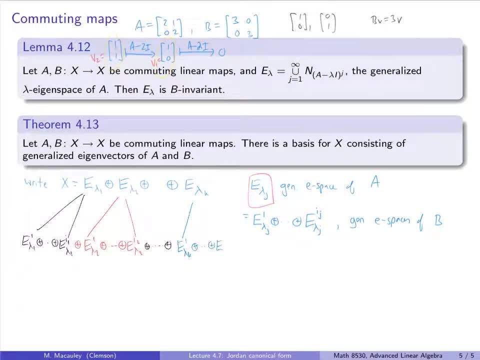 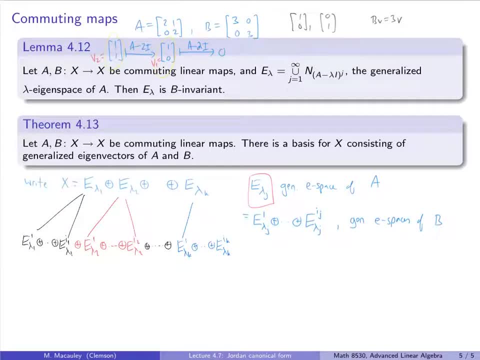 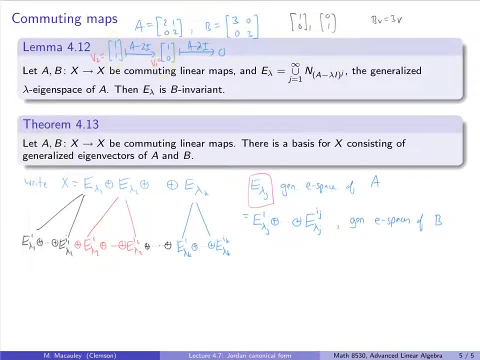 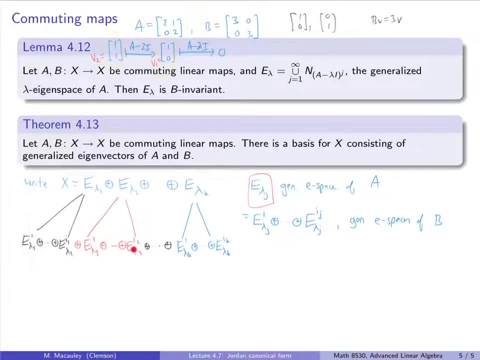 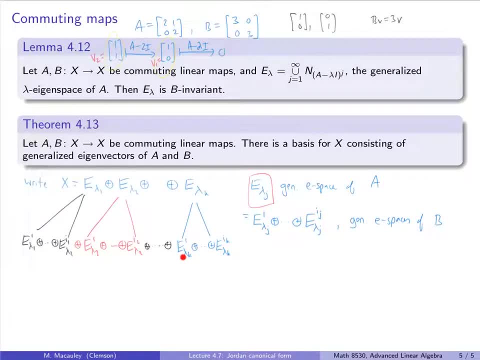 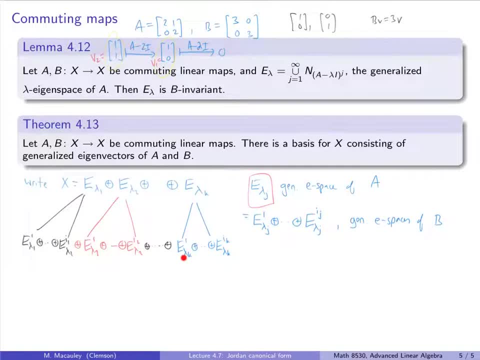 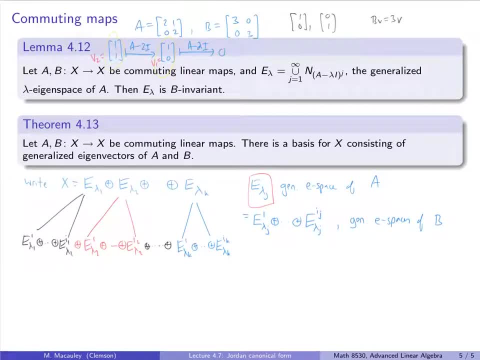 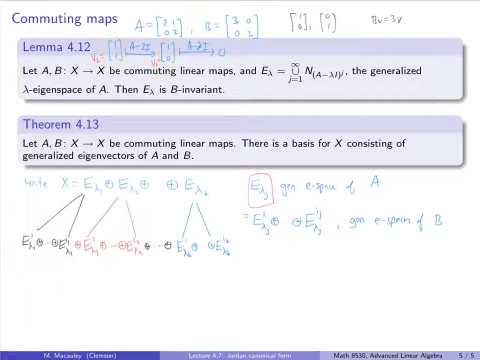 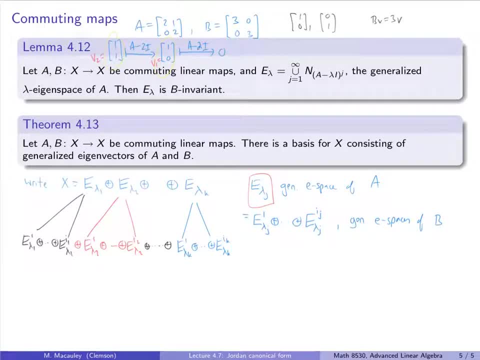 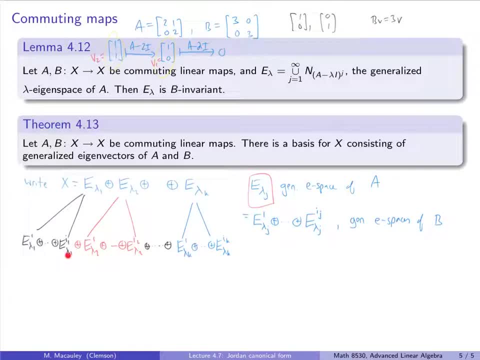 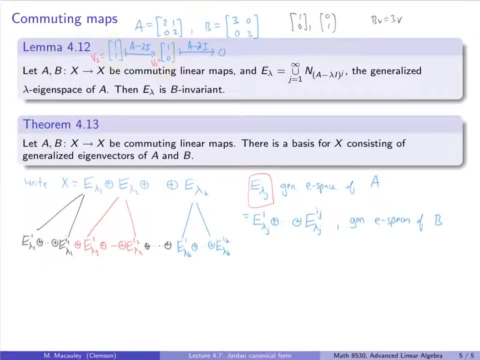 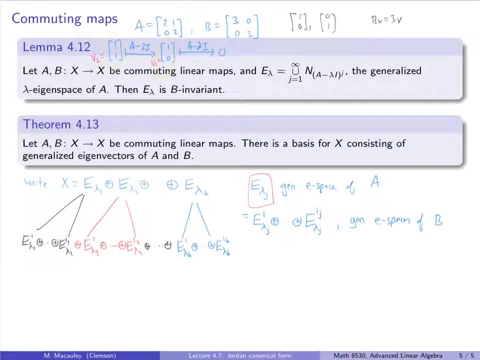 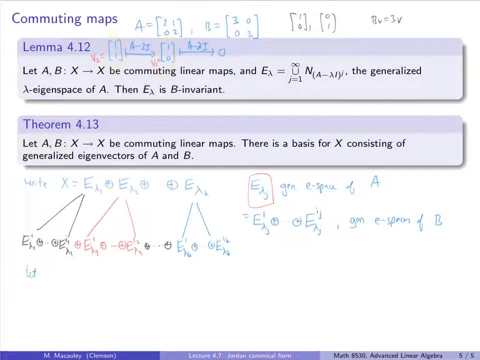 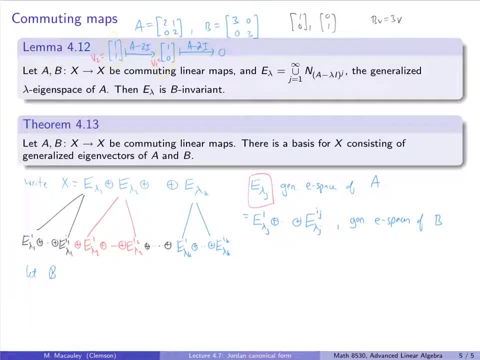 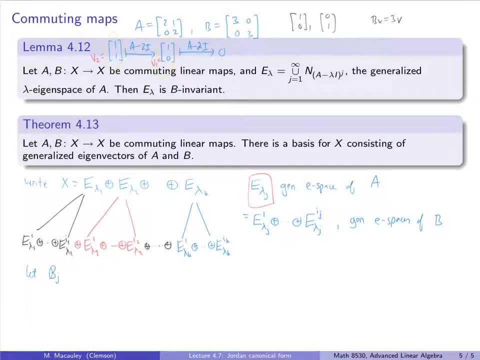 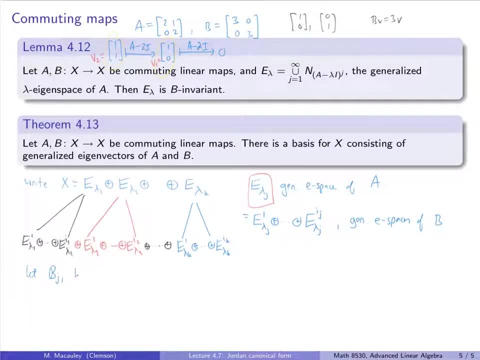 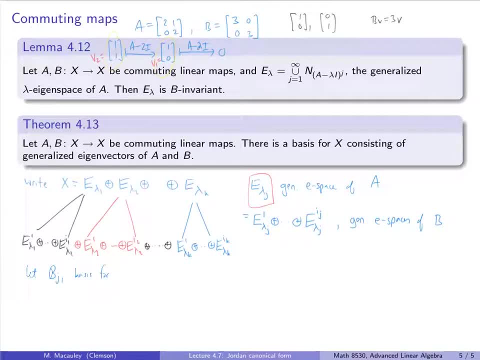 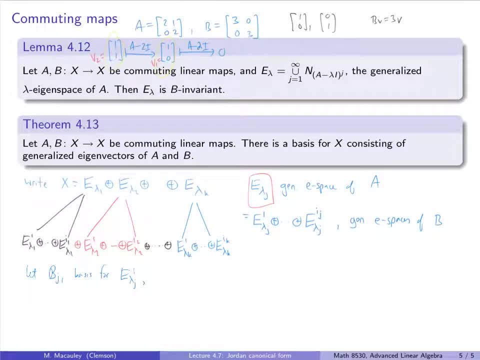 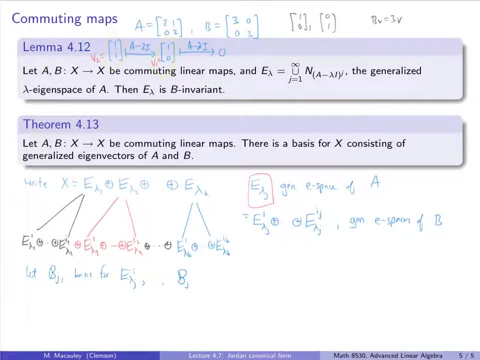 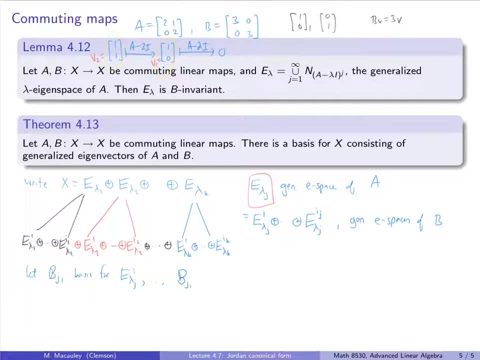 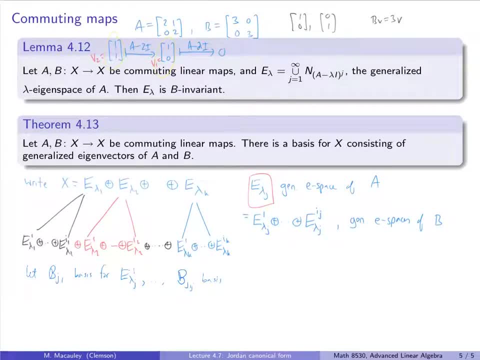 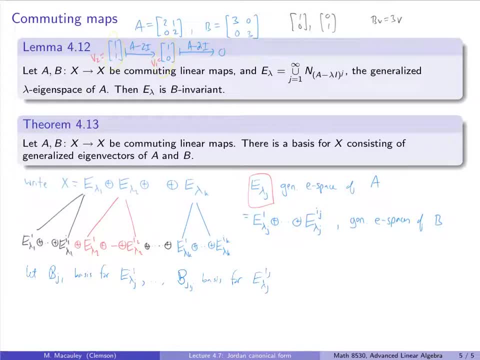 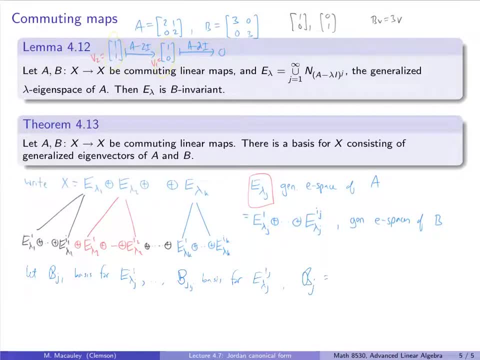 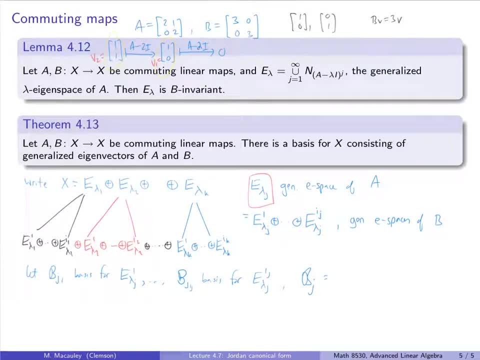 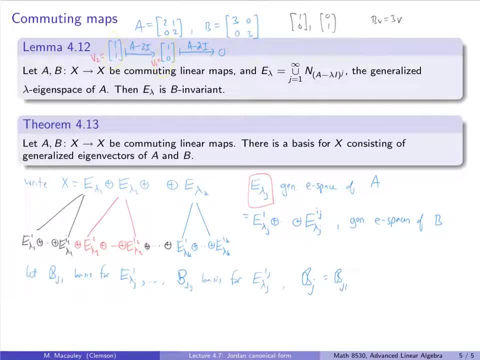 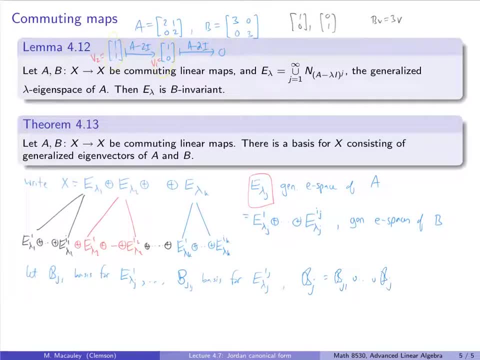 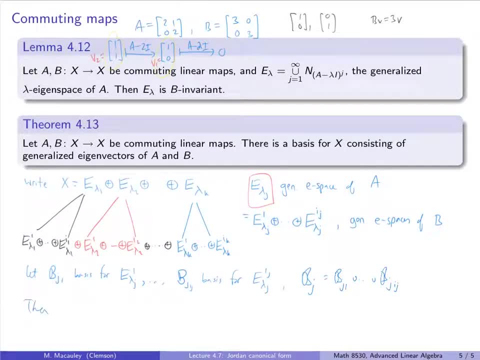 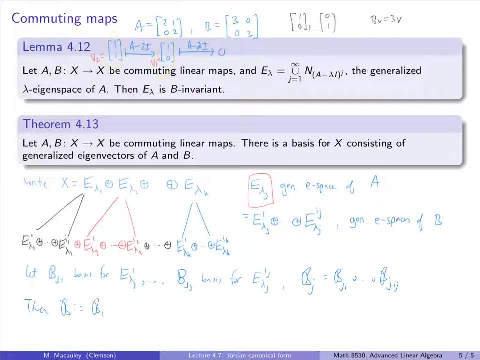 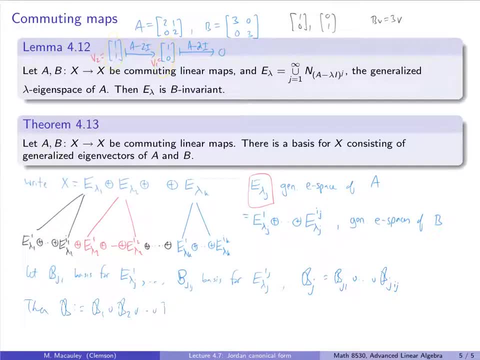 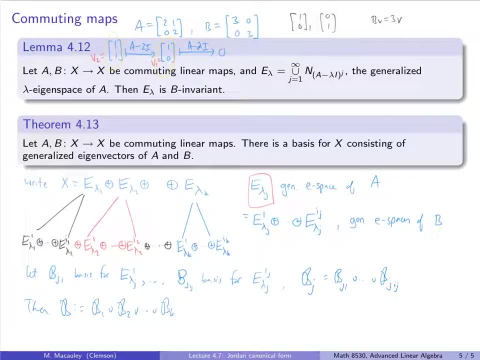 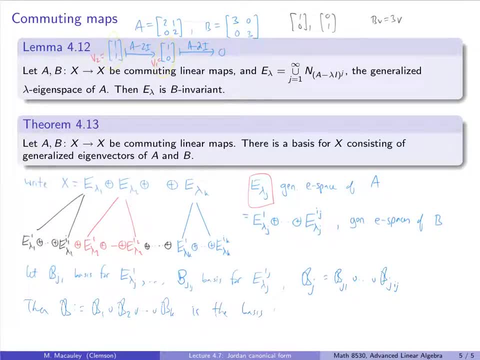 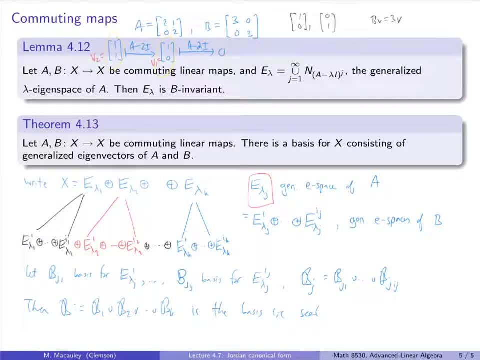 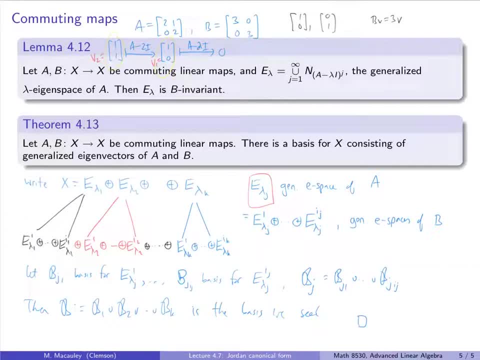 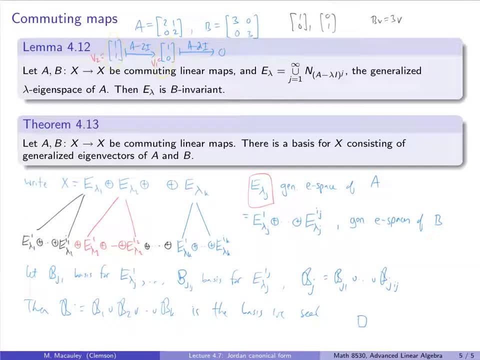 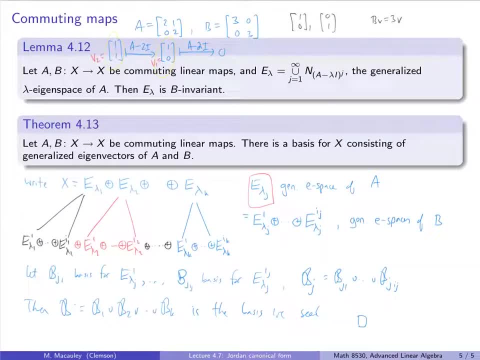 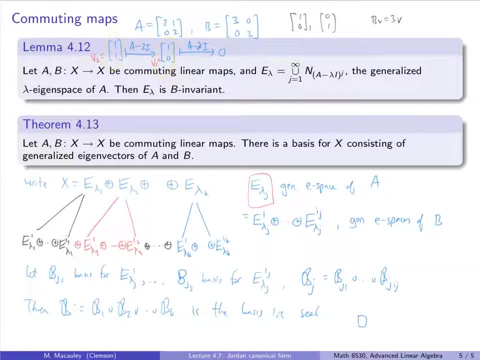 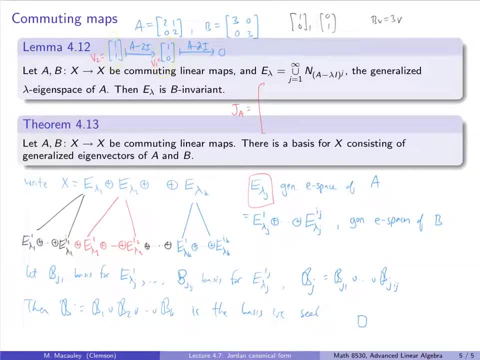 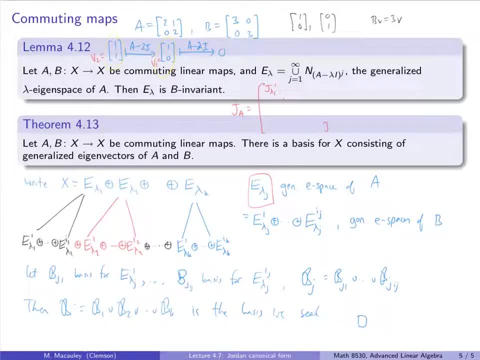 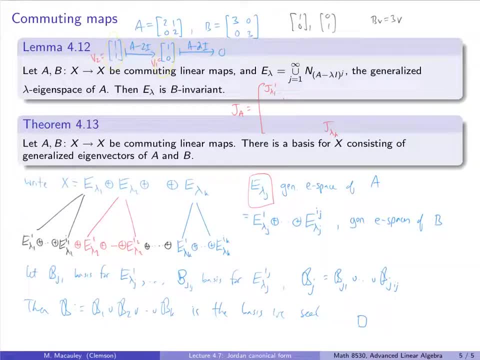 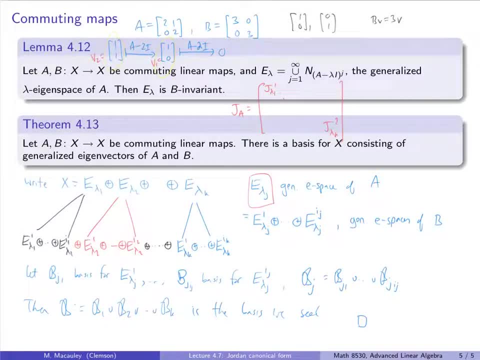 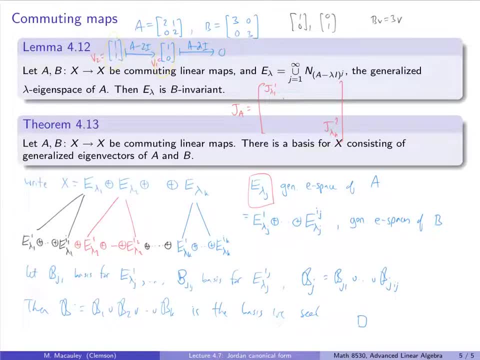 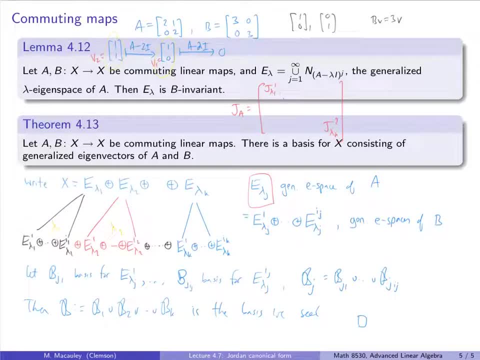 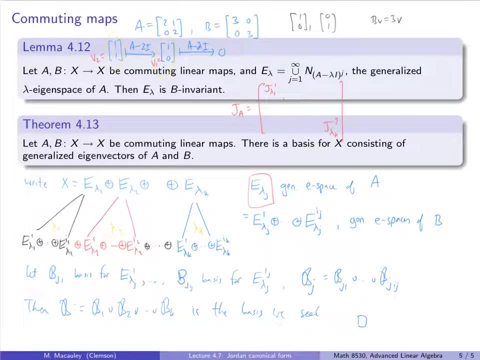 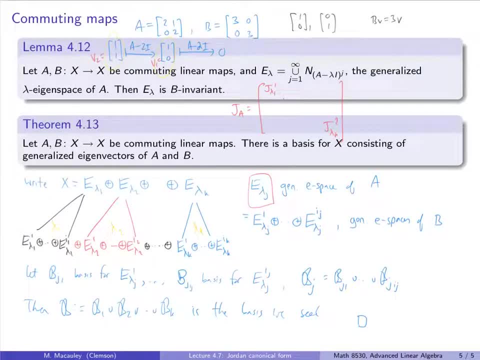 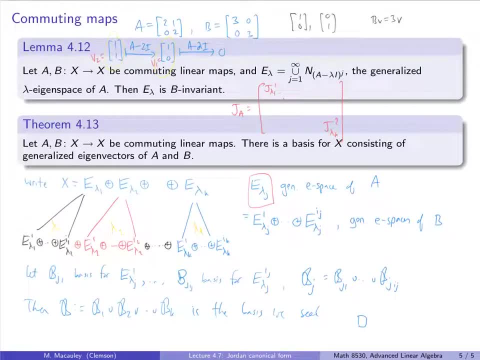 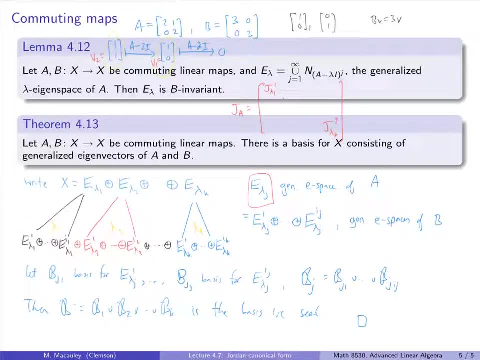 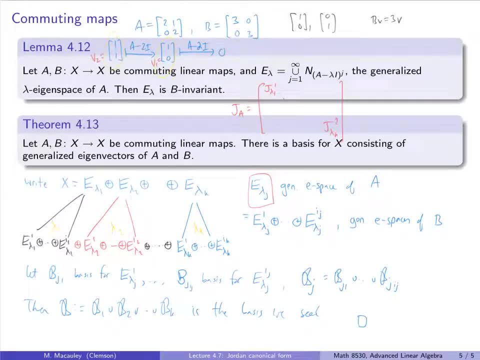 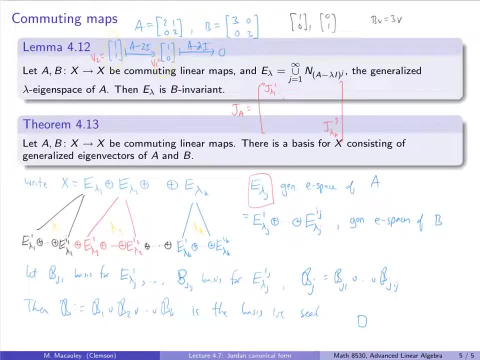 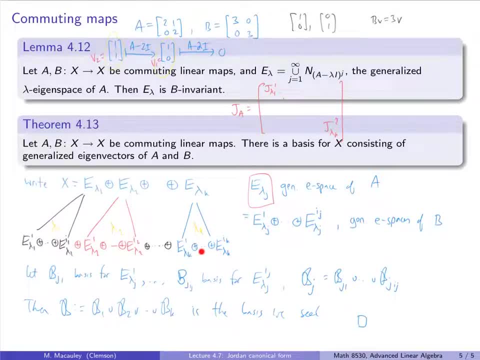 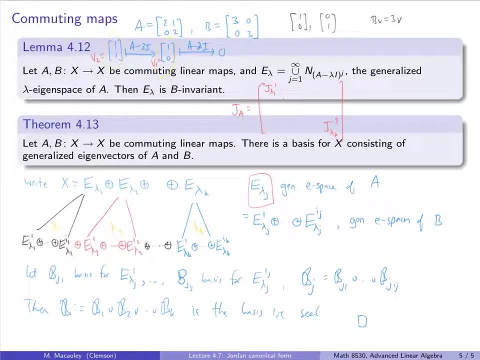 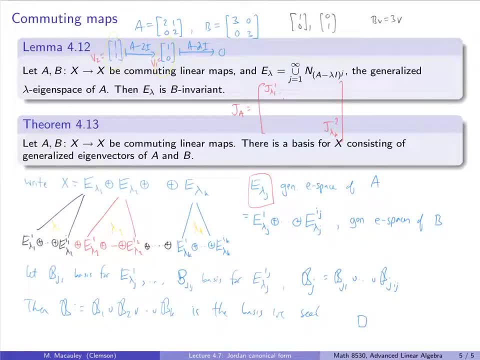 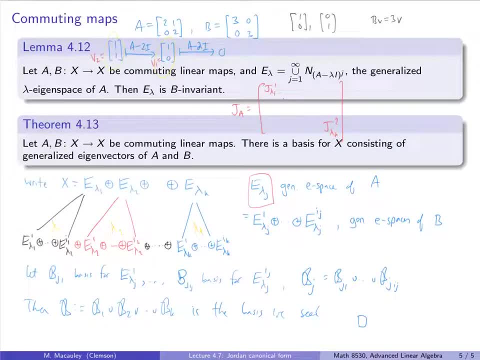 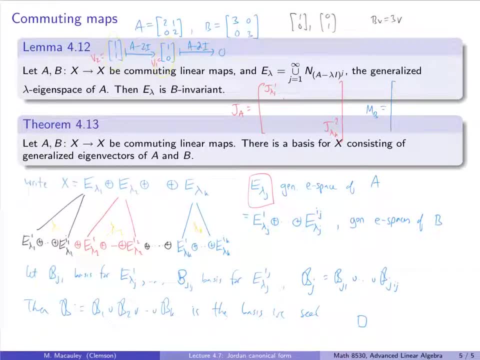 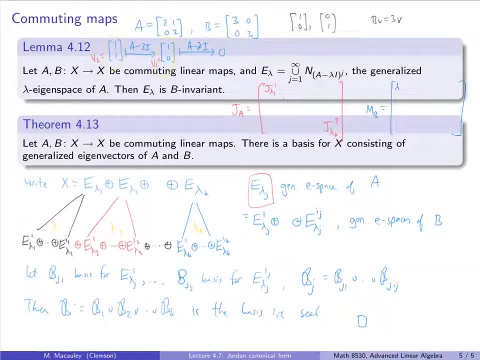 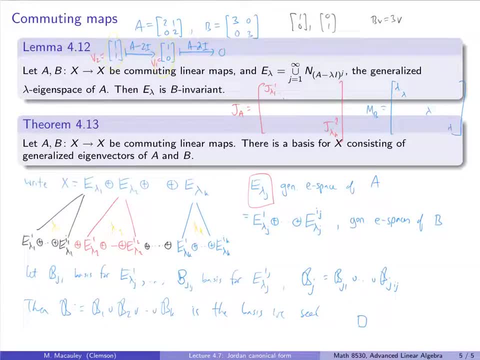 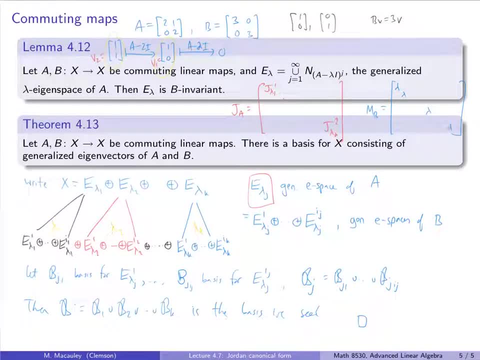 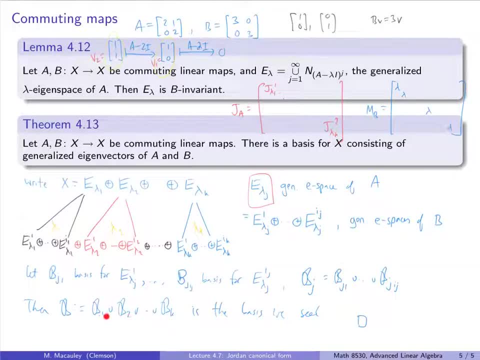 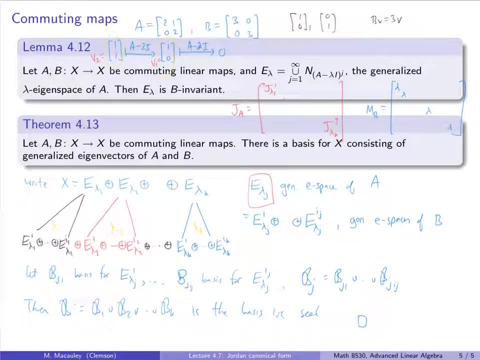 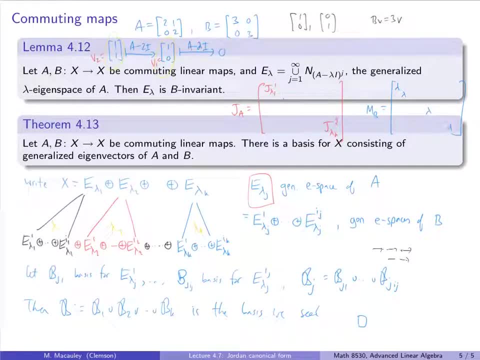 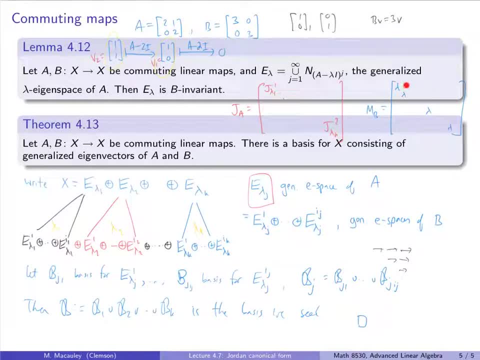 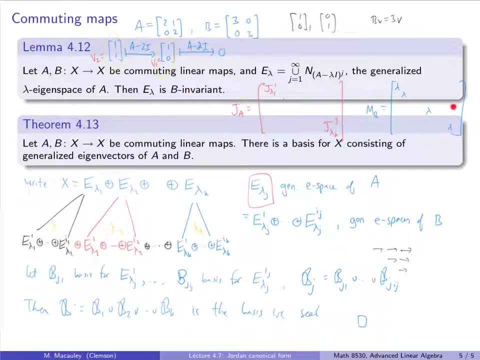 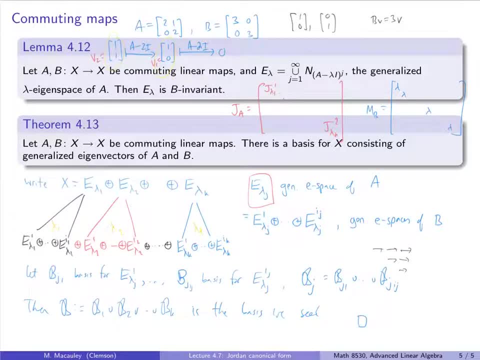 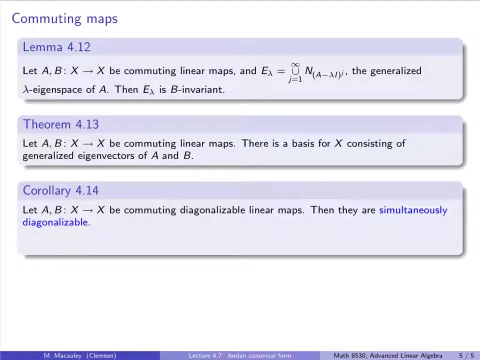 And let's be clear that E lambda j is a generalized eigenspace- one corollary of this, which you will see actually probably a lot more frequently than the statement itself, because it's something you can do in an undergraduate algebra course when you don't.